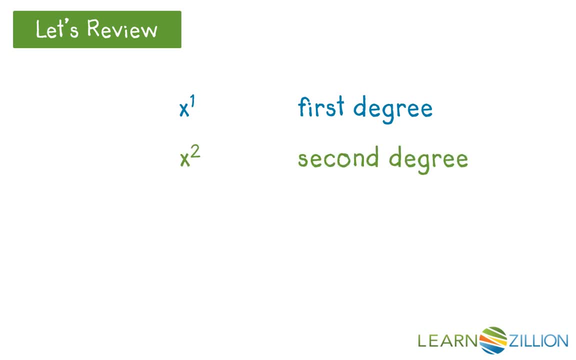 A second degree term would have an exponent of 2, and so forth. A common misunderstanding is that x cubed plus x squared equals x to the fifth. x cubed plus x squared involves adding, but x to the fifth is all multiplication. 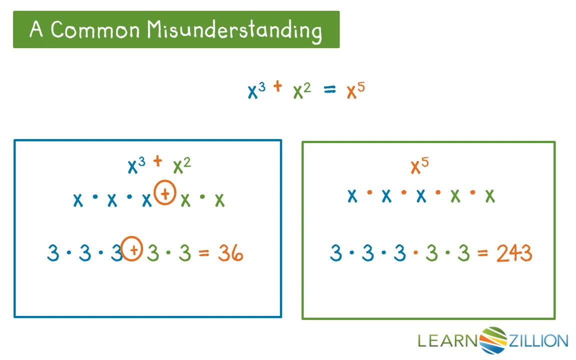 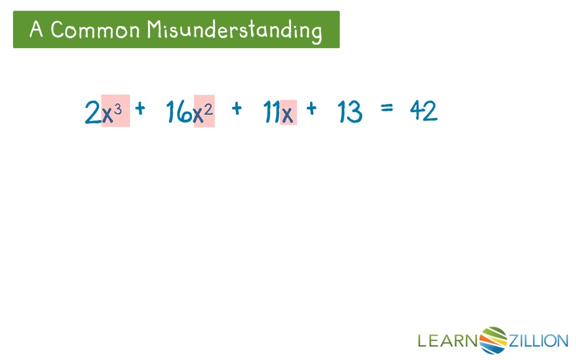 For example, for any value of x except zero, x cubed plus x squared will have a different value than x to the fifth. x cubed plus x squared equals x to the fifth. Neither can you add all the coefficients and all the exponents. 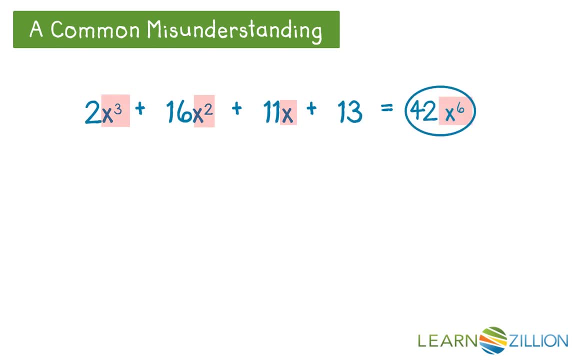 to get one combined term, Since the exponents are different. we do not have 42 like items. Our answer has to be shown as a group of several terms and cannot be one final term. This is the form that we use to write polynomial sums, and you will learn why in this lesson. 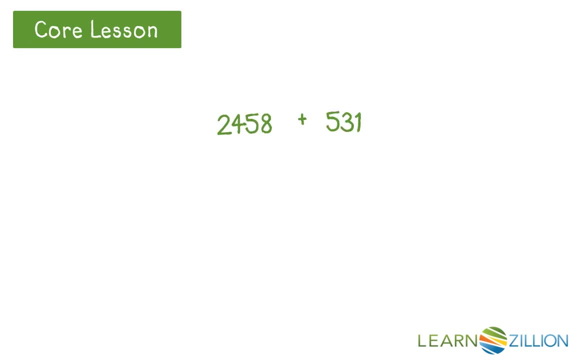 Let's compare adding 2,458 and 531 with adding these two polynomials. Just like we line up numbers by place value when we add, we would also line up exponential terms by degree when adding polynomials. 5x squared would line up under 4x squared because they are both second degree terms. 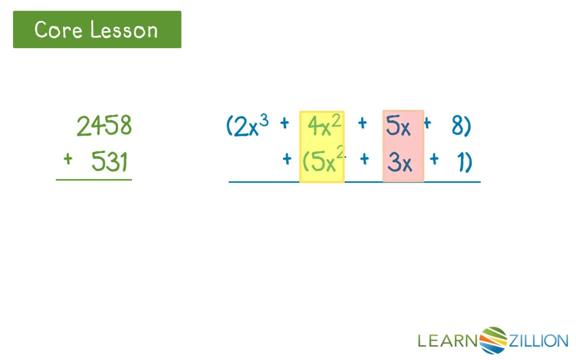 3x and 5x are both first degree terms and 8 and 1 are both ones units. Then, just as with whole numbers, we add the like terms. The sum would be 2x cubed plus 9x squared plus 8x plus 9.. 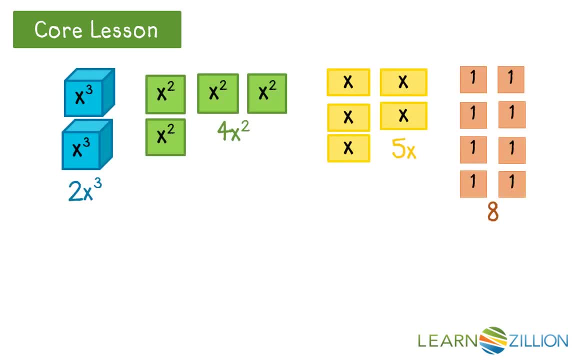 Let's look at this with algebra tiles. This represents 2x cubed plus 4x squared plus 5x plus 8. We add in the 5x squared plus 3x plus 1. We group the tiles by like shape. 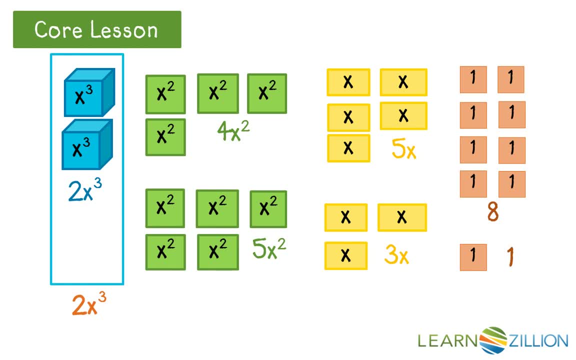 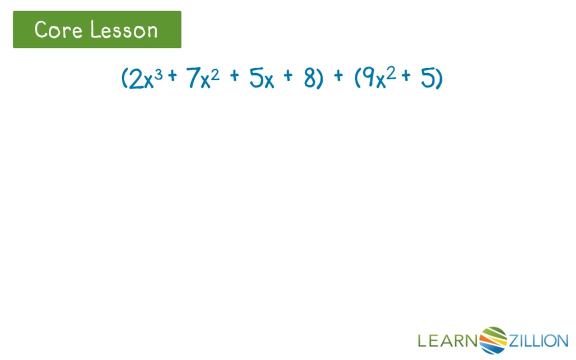 The result is 2x cubed. since no more were added, There are now 9x squared tiles, 8x's and 9 ones. Let's add polynomials that are a bit more complicated. There are no visible zeros to hold place value in polynomial expressions.